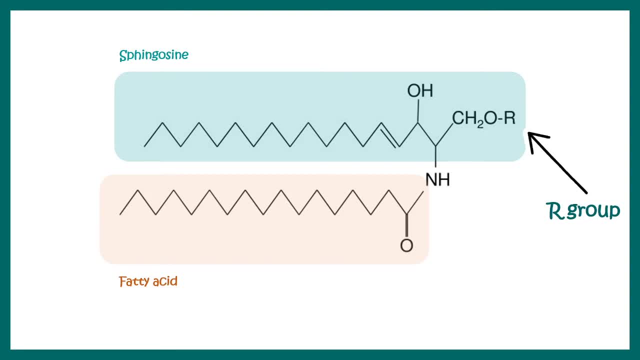 towards the R group. If this particular R group is hydrogen only, then this is known as ceramide. Now, if R group is glucose, then this particular sphingolipid would be known as cerebrosite and as the name suggests it. 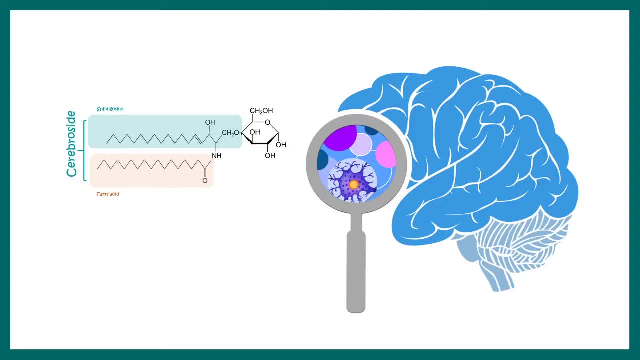 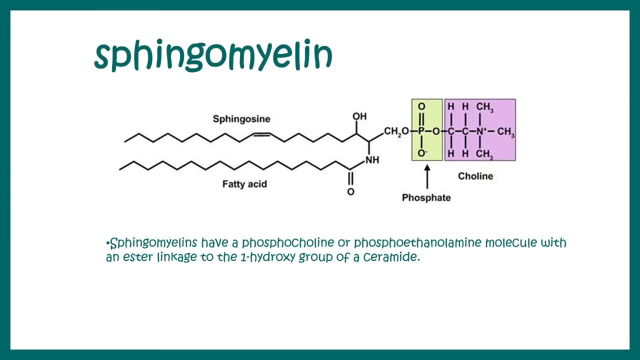 would be found in the nervous system, especially in the myelin shield. Then there is sphingomyelin, where the R group is phosphatidylcholine, And this is also considered as a phospholipid, but the difference is that they're both Hani to a formal Phospho. All right, let's pick up the case and ours Winnie, we'll filter her and let'sいきます the Phosph tease. 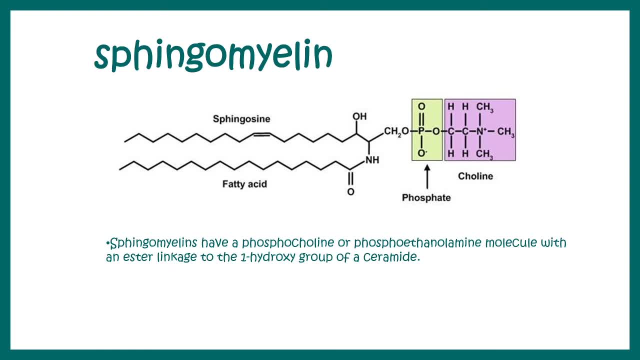 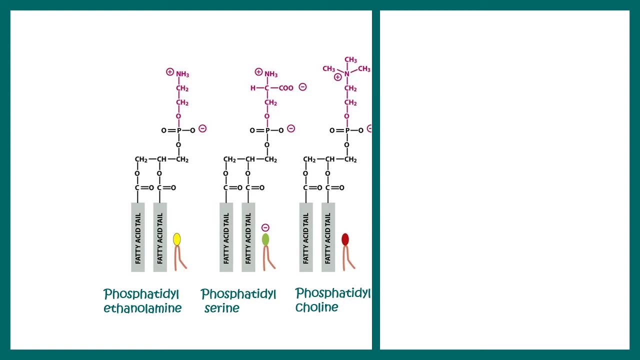 it doesn't have the glycerol moiety as the alcohol part. It is generally found in axons and myelin sheath. Especially, it is enriched in nervous system. So just to give you a quick comparison: phosphatidylcholine, serine or ethanolamine are characteristic phospholipids found in plasma. 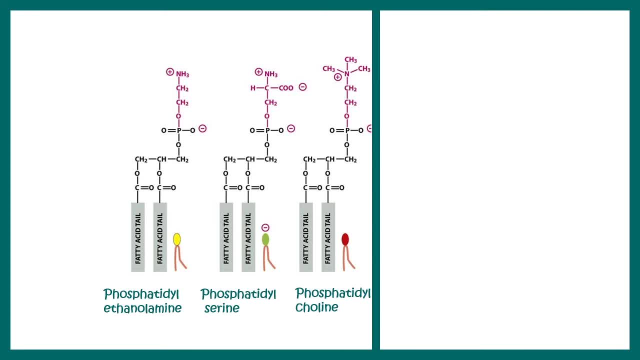 membrane. Now, phosphatidylcholine is not very different from a sphingomyelin. The only difference is it has a sphingosine moiety. So this sphingosine moiety makes sphingomyelin very different from phosphatidylcholine, and it is found in axons. Now let us talk about how these sphingolipids 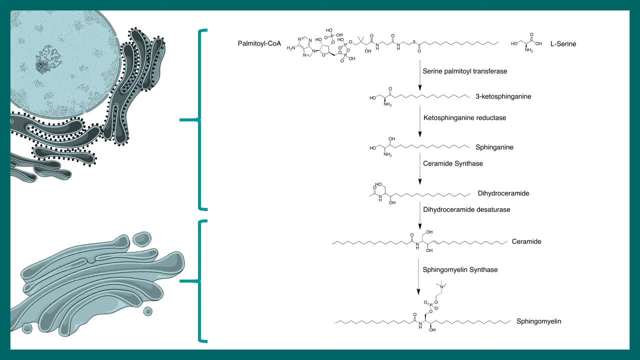 are synthesized. Sphingolipids are synthesized from pametoyl-CoA and L-lysine, and the enzyme serine-pametoyl transferase is the key commitment enzyme in this pathway and ultimately it forms 3-ketophosphinogeny and ultimately it leads to formation of ceramides. Ceramide synthesis takes 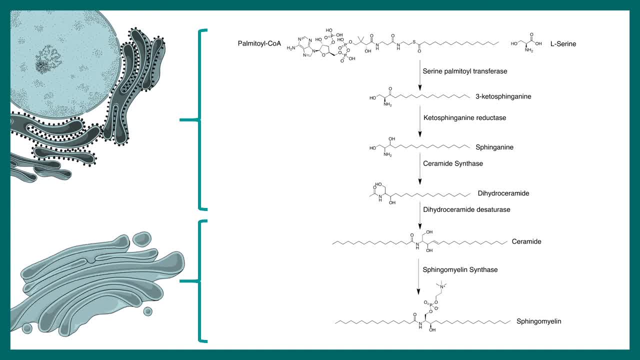 place in the endoplasmic reticulum Beyond ceramide. the further modification such as adding of some sugar moieties or other groups that takes place. or let's add addition of phosphatidylcholine group. these kind of things are happening in the endoplasmic reticulum. 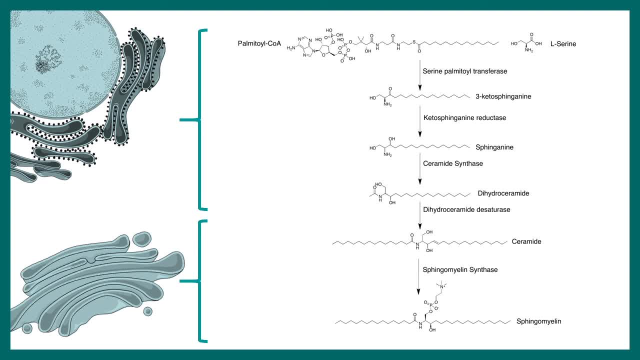 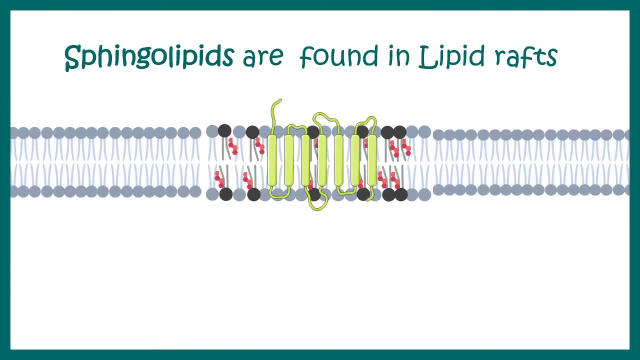 Golgi apparatus. So in a combination of golgi apparatus and endoplasmic reticulum, the synthesis of sphingolipids takes place. Sphingolipids are majorly found in lipid wraps. Lipid wraps are dense portion in the plasma membrane which has wide variety of functions, such as signaling function.